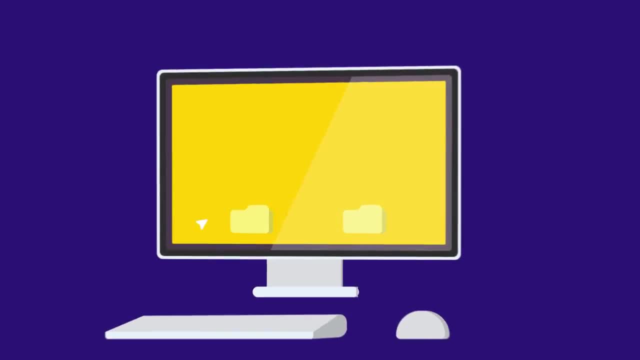 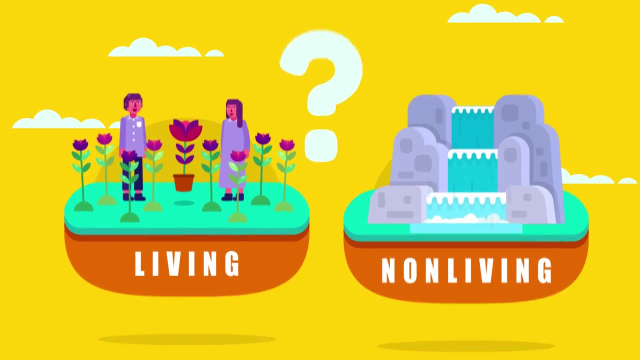 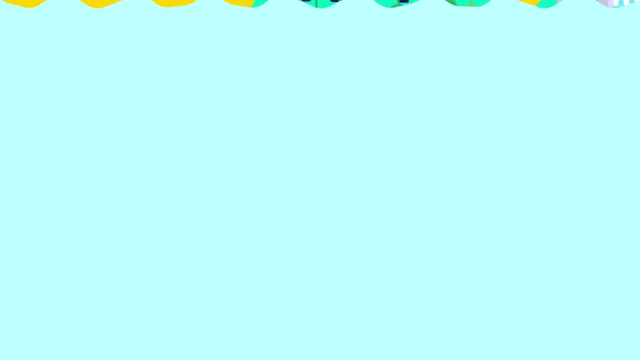 You may have learned to classify a rose or a human as living, rock and water as non-living. But why is this so? If you say that living is something that moves, but then flowing water can be called living, right, That's not entirely true. Life has a set of properties. 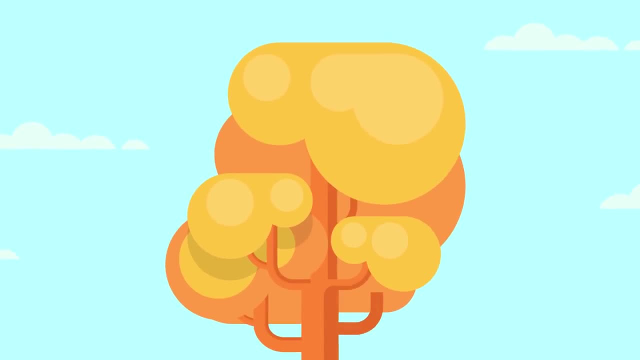 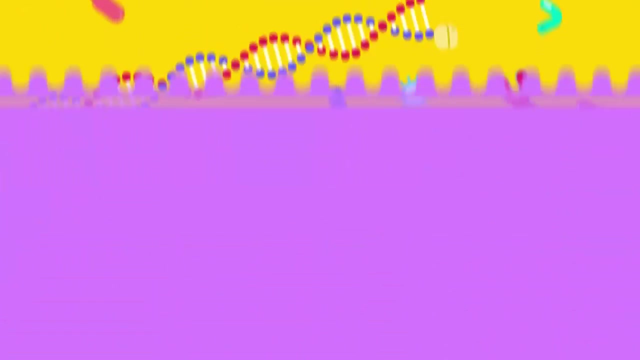 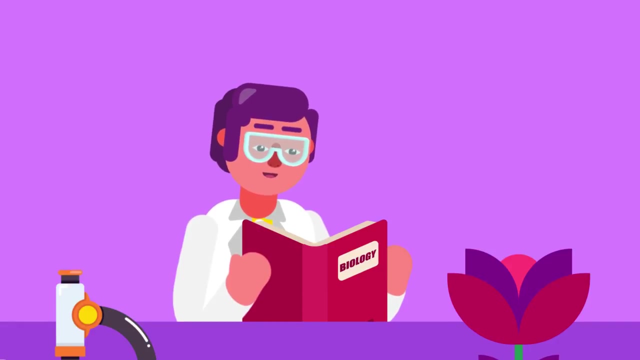 that an organism has to follow to be called living, And a wonderful discipline of science studies life in great detail. It is called biology. The word bio means living and logi means study. So biology means the study of living things. Simply put, anything which 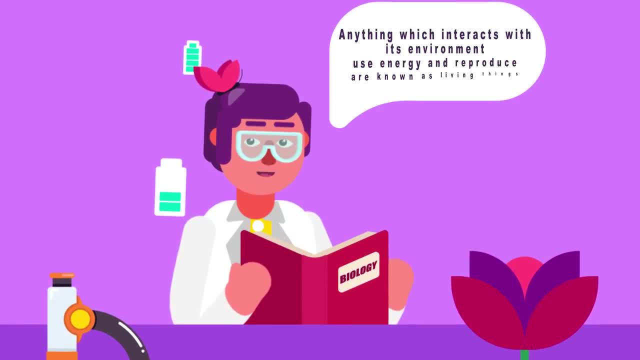 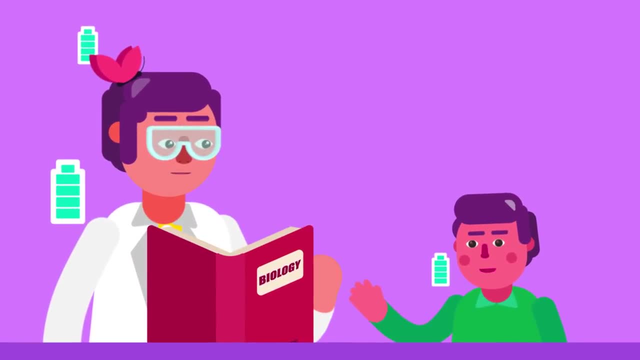 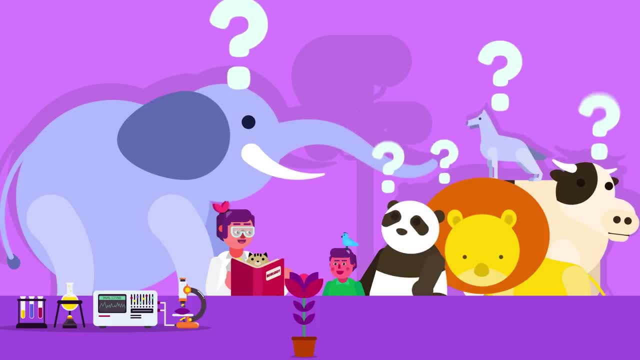 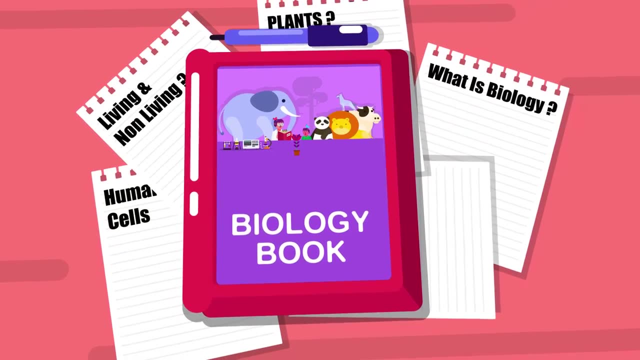 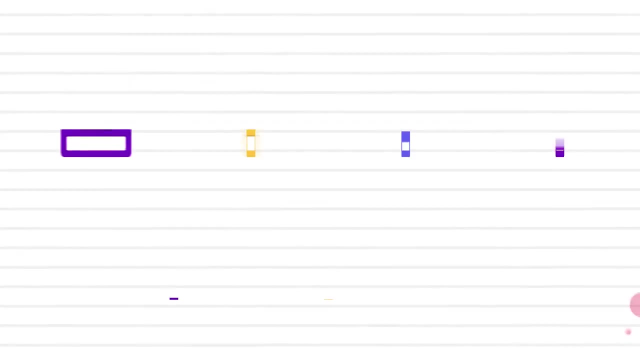 are all living organisms. Now the question arises: how many types of living things are there And how are they different from us? Biology is a field which answers these questions and many more questions related to living things. What is biology? There are 7 characteristics that a living thing follows, and therefore, 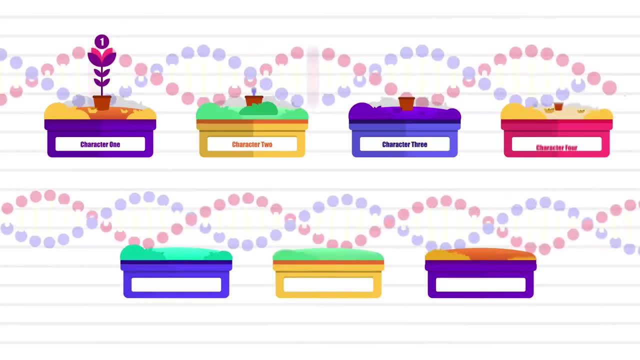 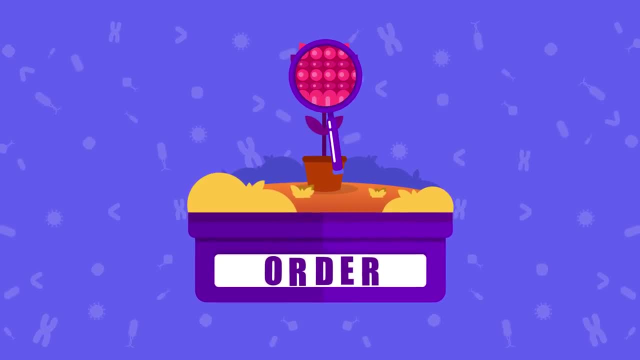 we study this in the vast field of biology. These are: 1. ORDER: If you examine a rose, you will notice it is very ordered. The petals are whirled around each other, with the center bearing seeds. This illustrates the highly ordered structure that typifies life. 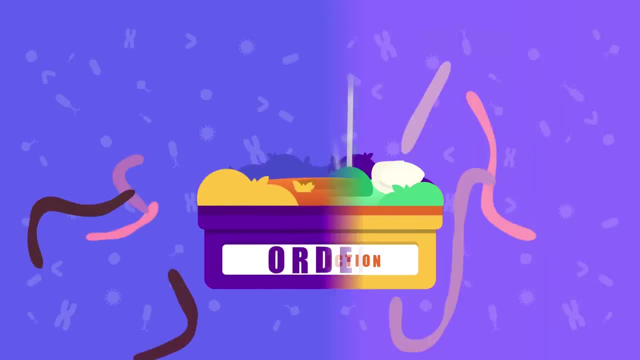 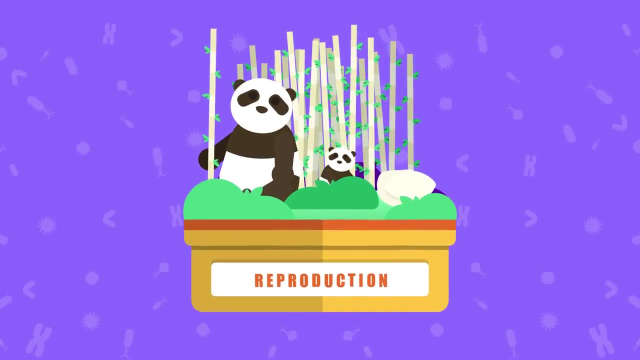 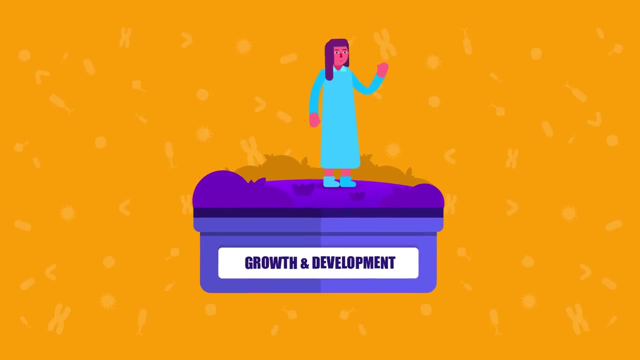 Living cells are the basis of this complex organization. 2. Reproduction: Organisms reproduce their own kind. A mother giant panda will always give birth to a panda, not a horse. We learned that from Kung Fu Panda too. 3. Growth and Development: Inherited information in the form of DNA. 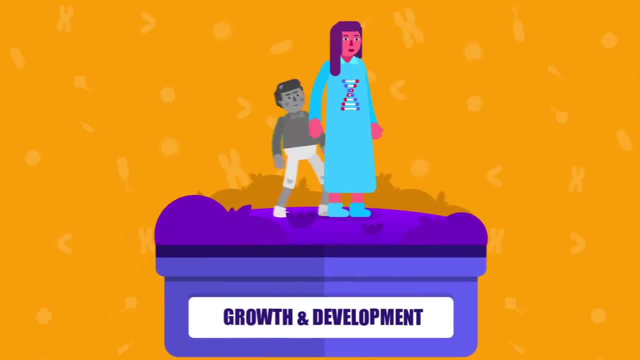 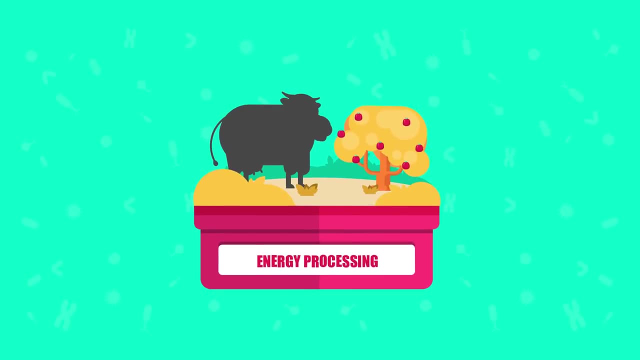 controls the pattern of growth and development of all organisms. You most probably look like your parents or a close relative thanks to the genes. 4. Energy Processing: We humans eat food to get energy. The food we eat has also eaten some food.